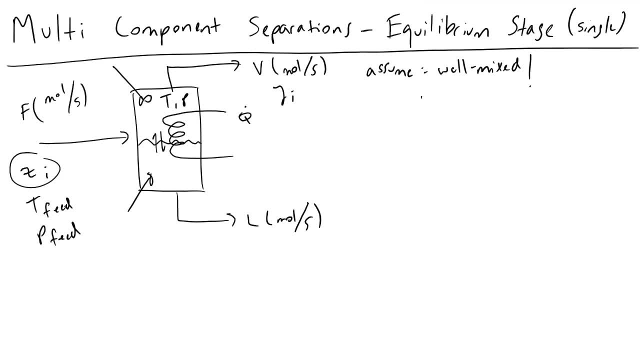 phases are well mixed And in practice, if you do a chemical operations lab, you will find that this is not the best assumption we can be making, because at the interface we'll find concentration gradients and the bulk fluid- either the bulk liquid or the bulk vapor phase- will have 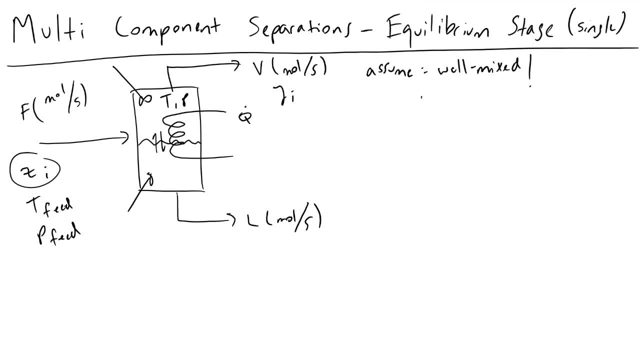 concentrations that are sometimes different. Quite often they'll be a little bit different from what that interfacial concentration is And therefore there will be a different driving force than what we think actually exists. But for the sake of an introduction to multiple 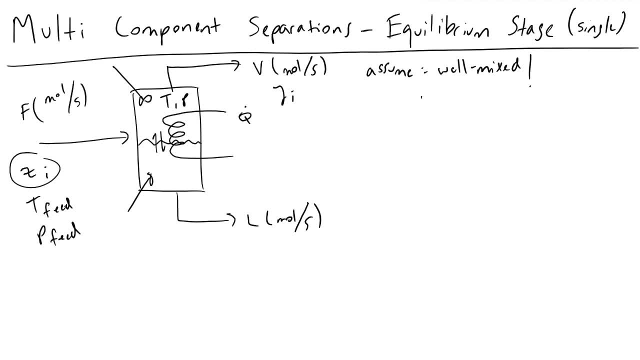 component distillations and equilibrium stages. we're going to make the assumption that we are well mixed And consequently, what that means is the concentration of our components, the molar ratios of our components and the vapor and liquid phase, And so, inside of our unit, we will pick a temperature and pressure to operate at, which is a big reason. 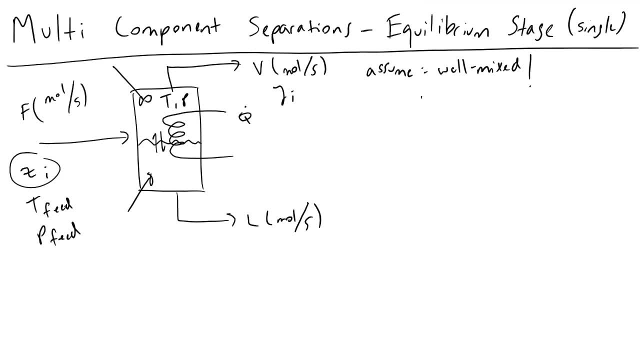 why we even care about writing all these equations and performing all these computer simulations And exiting our reactor. at the top will be our lighter components and they'll be leaving in our vapor phase with a flow rate of v moles per second, as well as a molar ratio of y sub i. 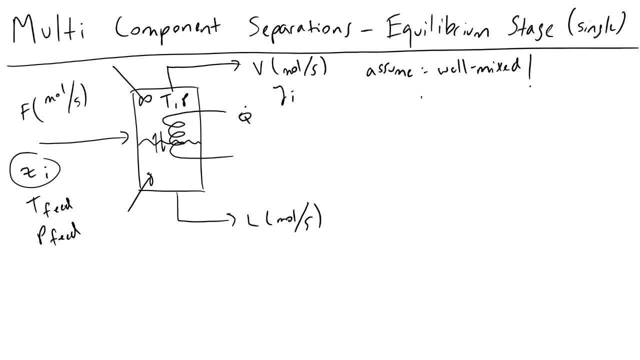 corresponding to each component. We will be adding heat or taking heat out, or maybe not adding any heat at all, but we may have q dot joules of energy being added per unit time, And so that's why I've written this variable q here, and this will appear in our enthalpy balance later on. 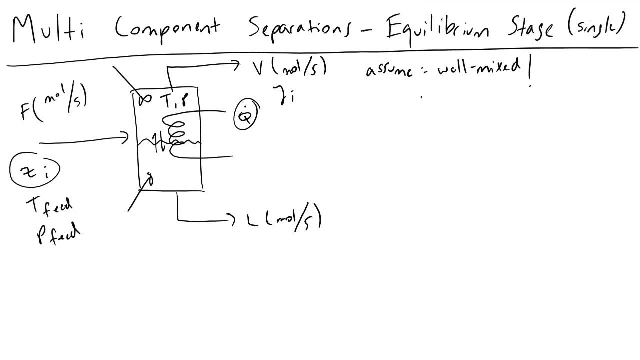 And then, exiting our equilibrium stage, we will have l moles per second, as well as x sub i, which is a molar ratio. And so the first question to ask is: how do we start figuring out? how many equations do you even need to fully define our system? And so, depending on the number of 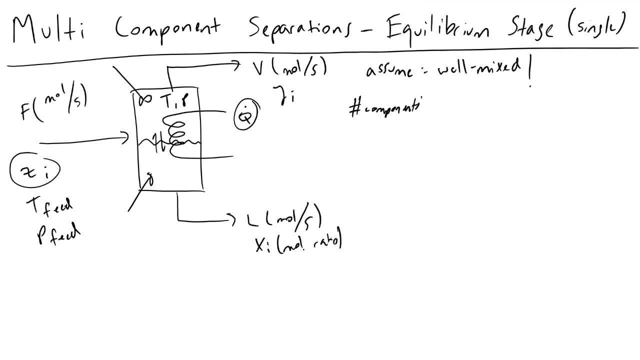 components we have. I'll let this be equal to k. k is an integer value, so just 5.. We will need- this is a number of unknowns that will exist- will be equal to 2k plus 4.. And so, if k was 5, that means there are 14 equations. 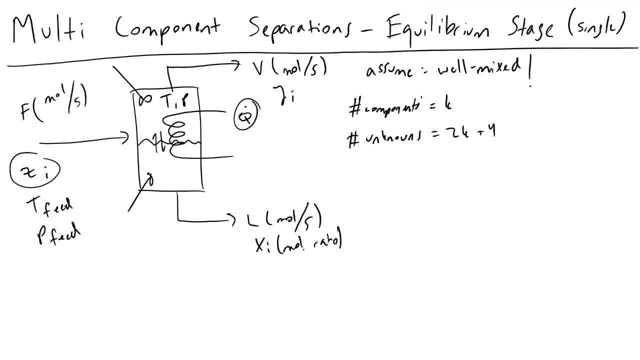 we're going to need to have to evaluate all 14 unknowns, And so the first equation that we're going to be able to create is a mole balance, or a component mole balance on each species inside of our reactor. And so what this tells us here? 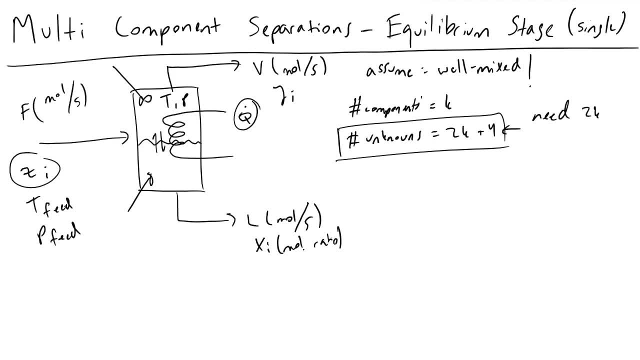 just to spell this out, is we need 2k plus 4 equations, And so equation 1 that we can derive is a component mole balance, And this tells us that because there's no, we're going to assume there's no reactions occurring, so the mole of each species will be conserved in our reactor. 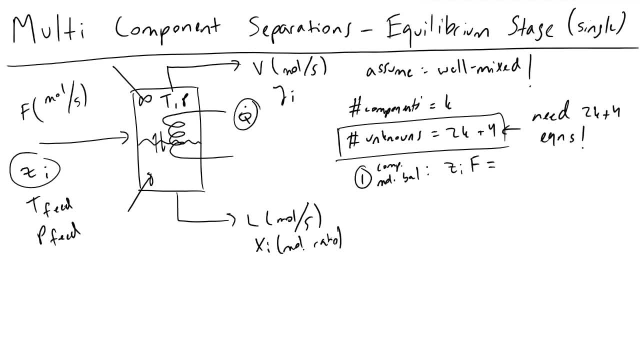 or not a reactor, but a partial. a total condenser is equivalent to y sub i times v plus x sub i times l, As well as the total number of moles entering must be equivalent to the total number of moles exiting. 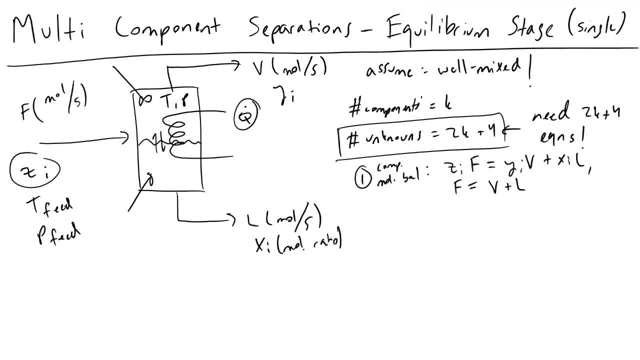 so f is equal to v plus l. This is the first set of equations that we can derive from our balance equations to fully define our system. The next set of equations we're going to get come from the fact that molar ratios must sum to unity, so the sum of the molar ratios. 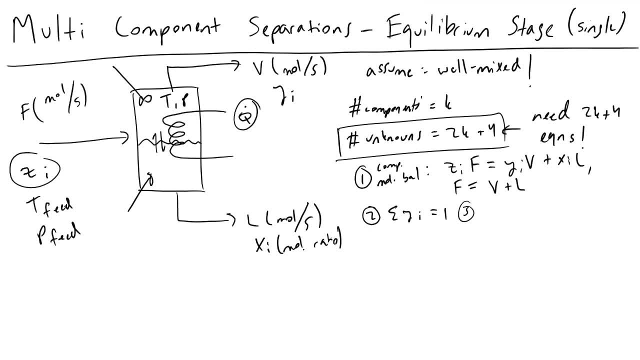 in your vapor phase must sum to unity, and the same can be said of the sum of the molar ratios in your liquid phase, X sub I, must also sum to unity, which is 1.. Next we're going to be turning to an enthalpy balance, and in our enthalpy 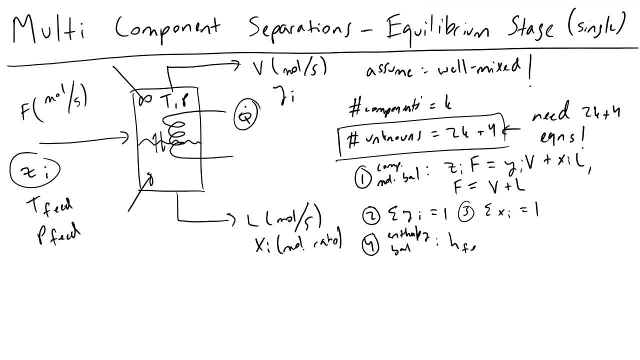 balance. what we will find is that the specific enthalpy of our feed times, F dot- and I want to spell this out- F dot has units of kilograms per second, because this is specific enthalpy- H sub feed, and I'll comment more on this later. 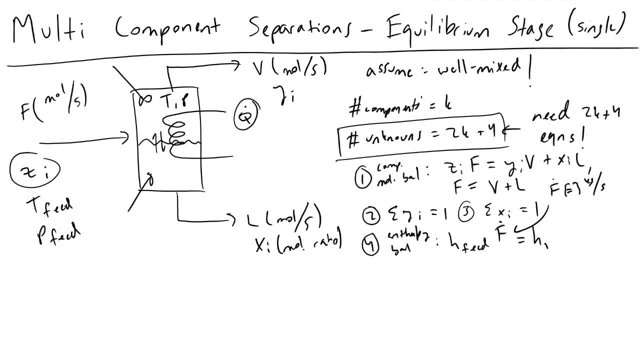 this is equivalent to the specific enthalpy of your vapor times, the mass flow rate of your vapor phase plus specific enthalpy of your vapor phase, plus specific enthalpy of your vapor phase, enthalpy of your liquid phase times, mass flow rate of your liquid phase. and. 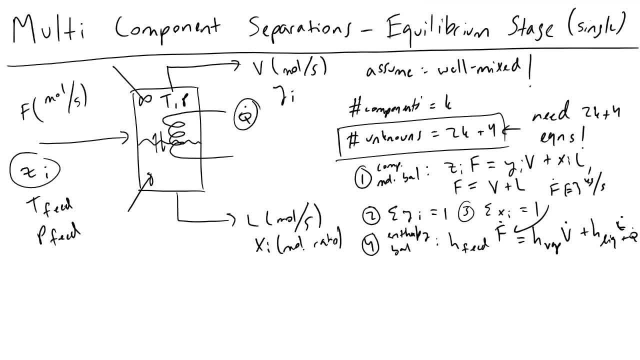 then plus Q dot. so if we're adding in moles of energy to our system, Q dot will have a positive value. if it's a refrigeration unit and we're taking moles out, Q will have a negative value in our enthalpy balance. next up we'll be 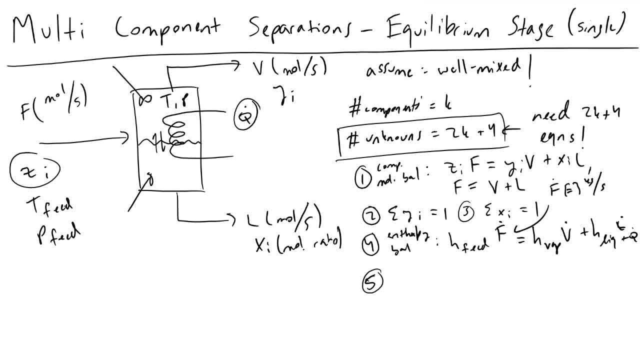 able to turn to our equilibrium relationship. we're going to be assuming that our equilibrium relationship we're going to be assuming that our partial condenser reaches equilibrium and therefore the concentration or the molar ratio of some component I in the vapor phase inside of our partial 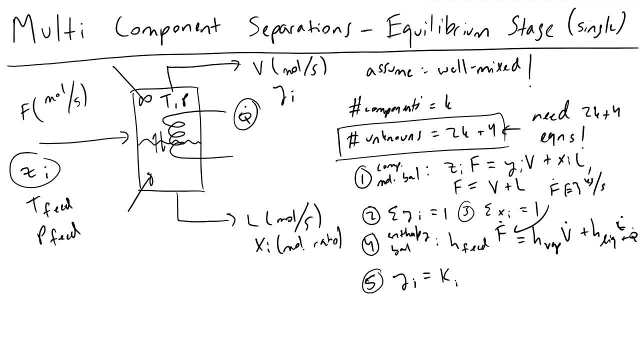 condenser must be related by some proportionality- constant case of I- to that same components, molar ratio within the liquid phase in our partial condenser. and again, if we're dealing with K components here, we're gonna have K equations because we're going to have a partial condenser and we're going to 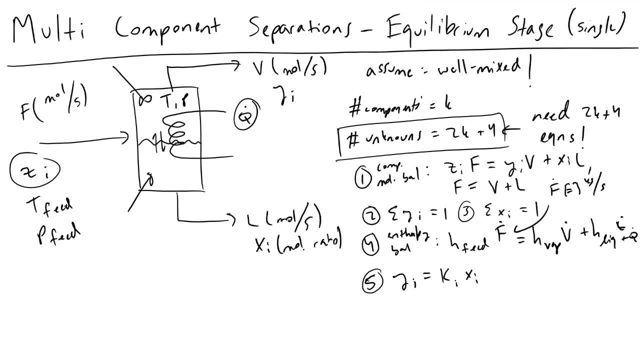 have a partial condenser, because it'll be like a number of equation be, some from K equations, because we're going to have a partial condenser and we're going to I could all of these, so you can, so you can hopefully see how much, how many. elevations we will get from all of these kind of mile-high perspectives, and so elevations we will get from all of these kind of mile-high perspectives, and so next up, the final equation or relation that we're going to be able to to assert in our analysis, is the fact that we need a pressure reduction predictor, mostly increaseded distance- surely depends on if I'm building on other rain storms out here, so maybe- which means the four times just represented in the squares, which then actually create a constant finance. 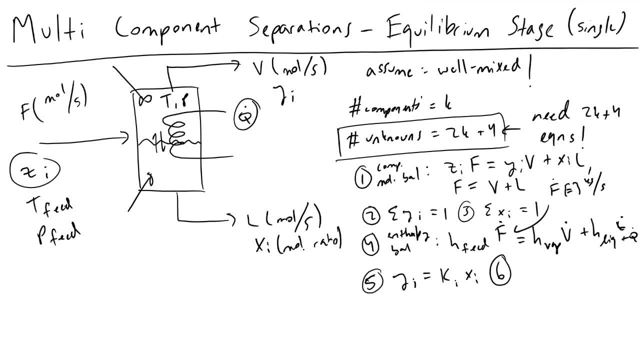 or furtherwan. it would be the other way around if I am building on a spin lines one way around, which means even smaller than a constant finance difference between our feed and whatever's inside of our partial condenser. In order to drive fluid flow, you need a pressure difference, much like in electricity, how you need a voltage potential to 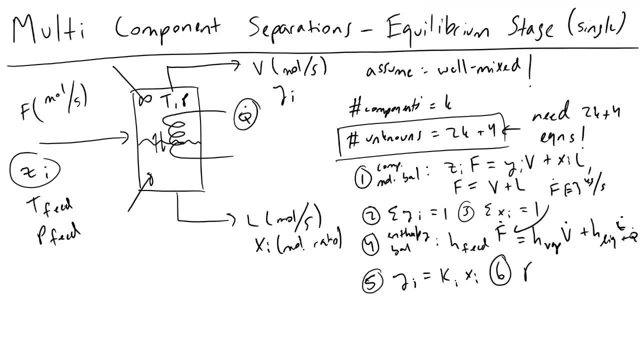 have a current, And what this tells us is that the pressure of our feed must be greater than the pressure that we operate our tank at. So if you have a higher pressure, our fluids will flow from areas of high pressure to low pressure. our feed will enter our tank. So this is the final. 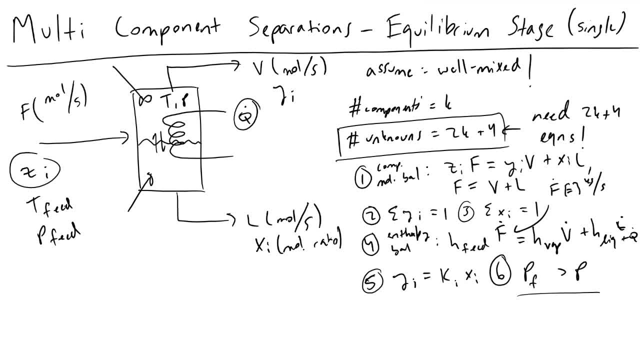 relation that we're able to demand in our partial condenser unit. And so, with that said, I'd now like to speak a little bit more about these specific enthalpy values that we saw here with this term here, So H feed is called specific. 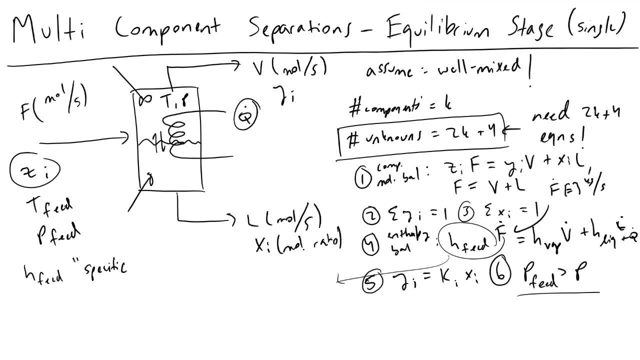 and specific is another way of saying per mass specific enthalpy of the feed And H sub feed, and the same can be said of all the other specific enthalpies. like the enthalpy of the specific enthalpy of the vapor phase is a function of 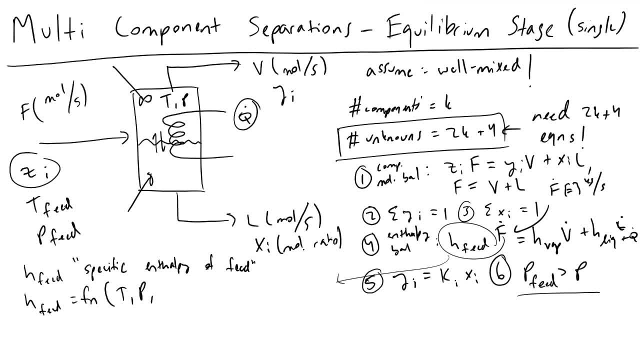 temperature, pressure and whatever other components are present. And this is because, as you learn in a thermodynamics course, depending on whether species are present in a mixture or solution, they can take on partial molar properties and new or slightly varied thermodynamic characteristics, So enthalpy. 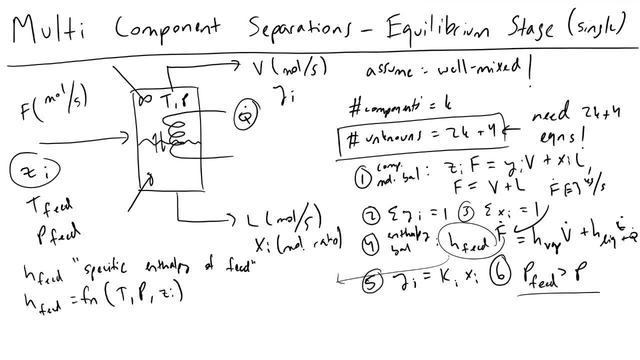 the specific enthalpy of your feed can be very tricky to calculate, So it will get a little bit more complicated, And it's another reason why we're going to talk about the specific enthalpy of your feed. And it's another reason why we're going to talk about the specific enthalpy of your feed, And it's another reason. 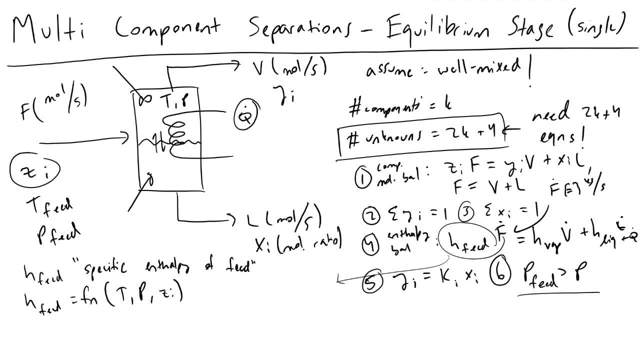 why doing these calculations by hand gets so tricky. But it can be done through tools like Aspen and or COMSOL. And another thing we can comment on here is this equilibrium relation that we see here with K sub i. K sub i, much like the specific enthalpy, is also a function. 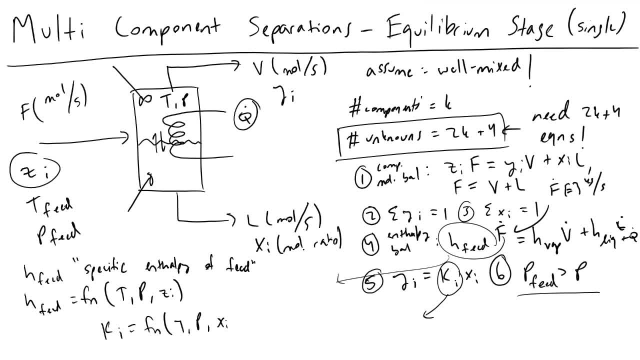 of temperature, pressure and what other components are also present in that solution. And so these are all handled by several equations, And if you take Aspen, for instance, they have a database where they obtain thermodynamic properties from NIST And with those thermodynamic